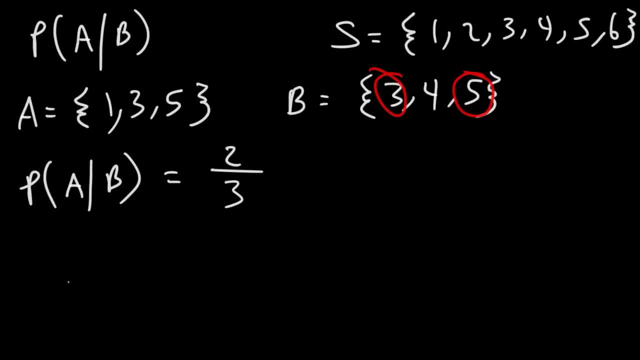 conditional probability. But now this is a formula that you need to know To calculate this conditional probability: it's the probability of event A and event B occurring divided by the probability that event B will occur. So what is the probability of getting event B? B has three outcomes that lead to it. 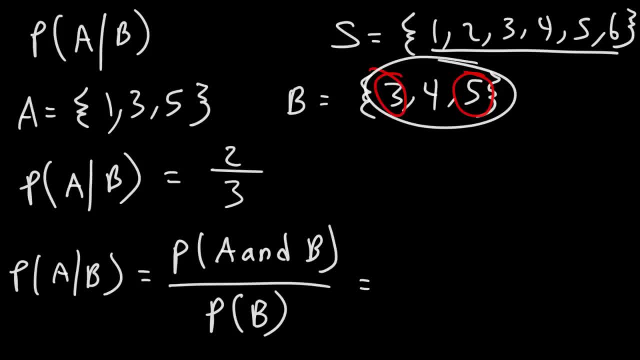 out of a total of six outcomes in a row. So what is the probability of getting event B? B is half of the number that will occur in the sample space. So when you roll a six-sided die there's six numbers you can get and B is half of those numbers. So the probability that event B 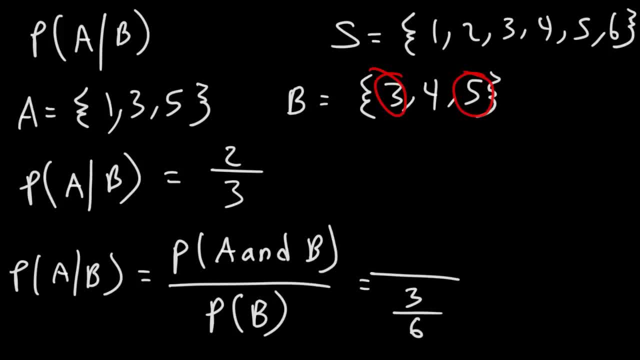 will occur is 3 out of 6.. Now what about the probability of events A and B occurring? Well, let's write the sample space for A and B. So this is the intersection of A and B, And we know that the numbers 3 and 5 are the same number. So we know that B is half of the number that will occur. 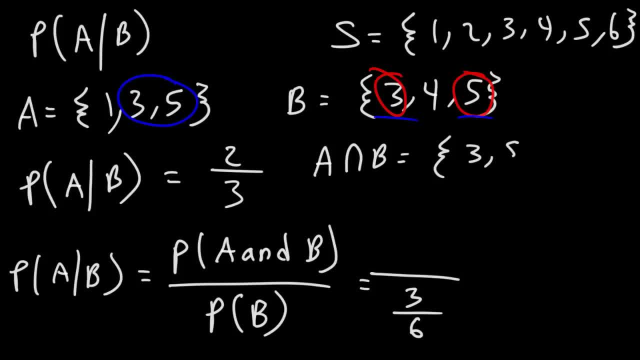 corresponds to a and b. so event a and b will occur if we get two numbers out of the six potential numbers that we could get. so the probability of a and b occurring is two over six. now to simplify this complex fraction, let's multiply the top and bottom by six so that the number six will cancel. 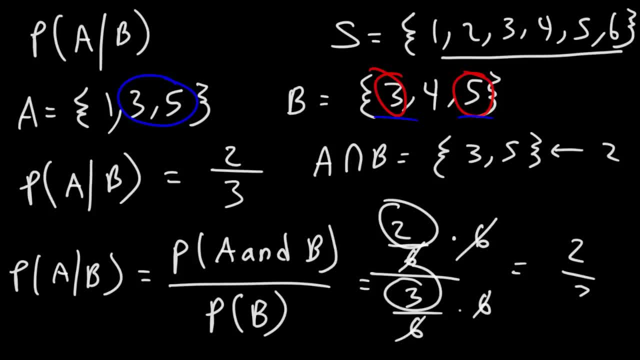 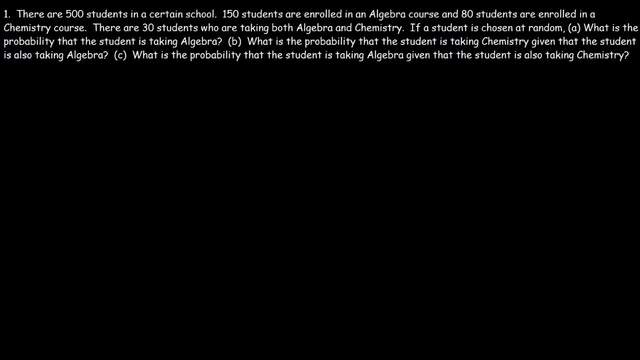 and so we're left with two over three, which is the same as what we see here. so that's a simple way in which you can calculate the conditional probability of an event occurring. but now let's look at some more example problems. there are 500 students in a certain school. 150 students are enrolled in an algebra course. 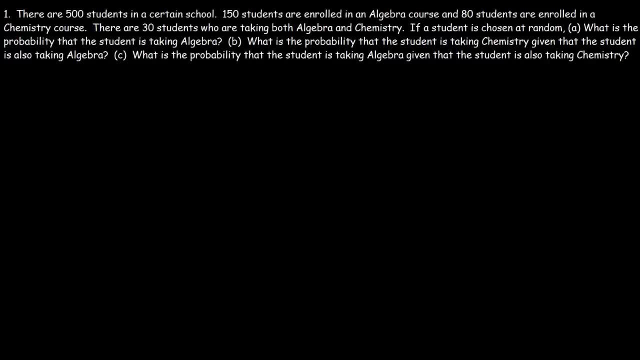 and, and and students are enrolled in a chemistry course. There are 30 students who are taking both algebra and chemistry. If a student is chosen at random, what is the probability that the student is taking algebra? Before we begin, let's draw a Venn. 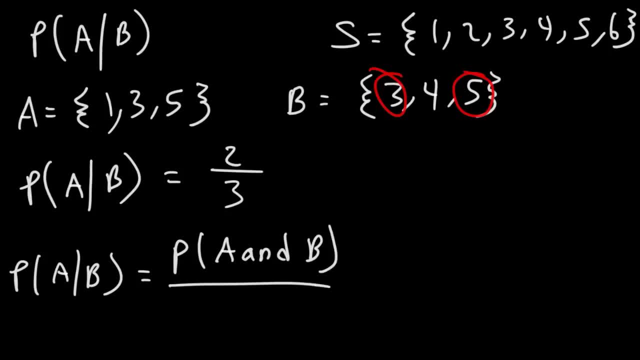 and event B occurring, divided by the probability that event B will occur. So what is the probability of getting event B? B has three outcomes that lead to it out of a total of six outcomes in B, the sample space. So when you roll a six-sided die there's six numbers you can get and B is 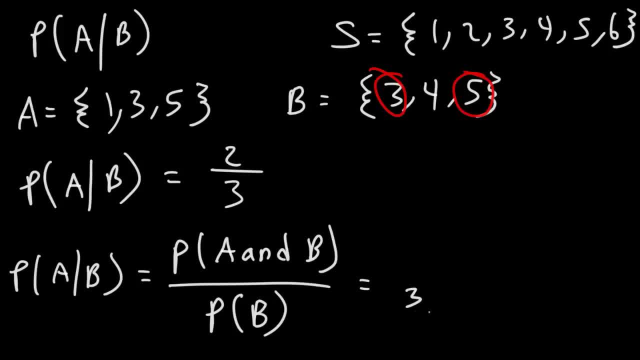 half of those numbers. So the probability that event B will occur is 3 out of 6.. Now, what about the probability of events A and B occurring? Well, let's write the sample space for A and B. So this is the intersection of A and B, and we know that the numbers 3 and 5 corresponds to A and B. 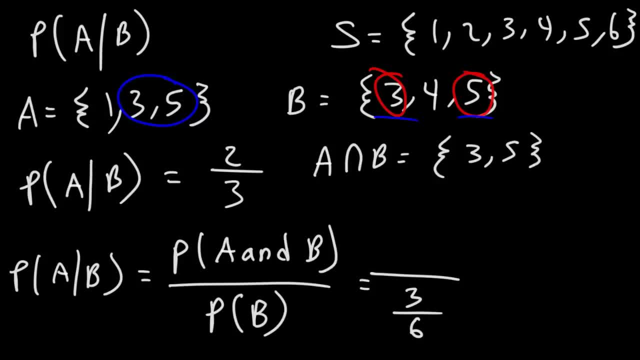 So event A and B will occur if we get two numbers out of the six potential numbers that we could get. So the probability of A and B occurring is 2 over 6.. Now to simplify this complex fraction, let's multiply the top and bottom by 6.. 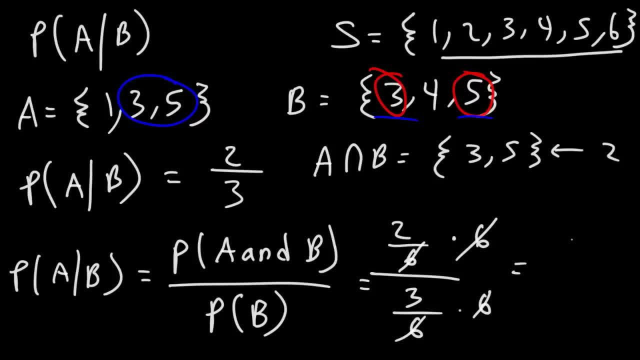 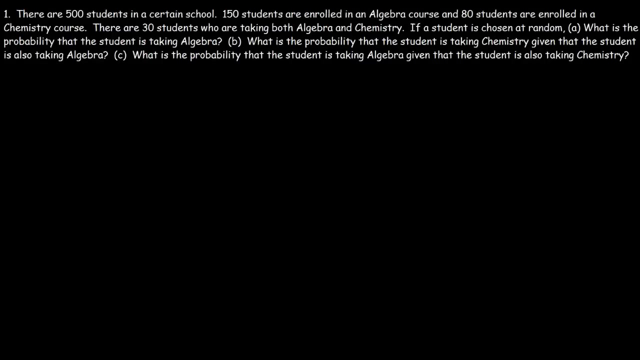 So that the number 6 will cancel, And so we're left with 2 over 3, which is the same as what we see here. So that's a simple way in which you can calculate the conditional probability of an event occurring. But now let's look at some more example problems. There are 500 students in a certain 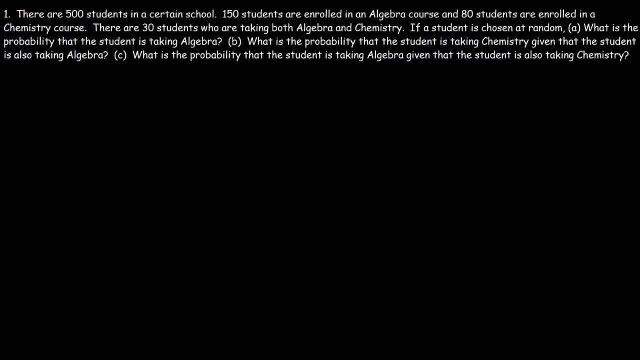 school, 150 students Are enrolled in an algebra course And 80 students are enrolled in a chemistry course. There are 30 students who are taking both algebra and chemistry. If a student is chosen at random, what is the probability that the student is taking algebra? 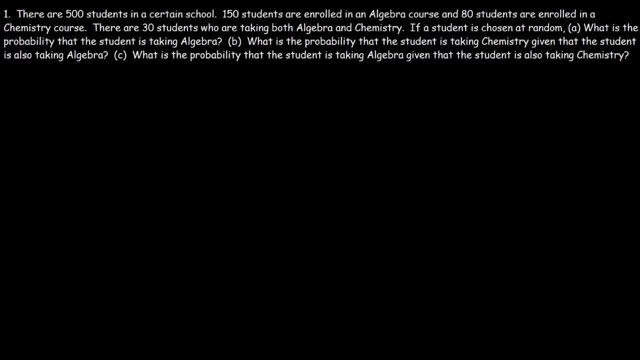 Before we begin, let's draw a Venn diagram. So we're going to draw a Venn diagram. So we're going to draw a Venn diagram. So we're going to draw two circles, with the circles intersecting each other. Let's put A for algebra and C for chemistry. 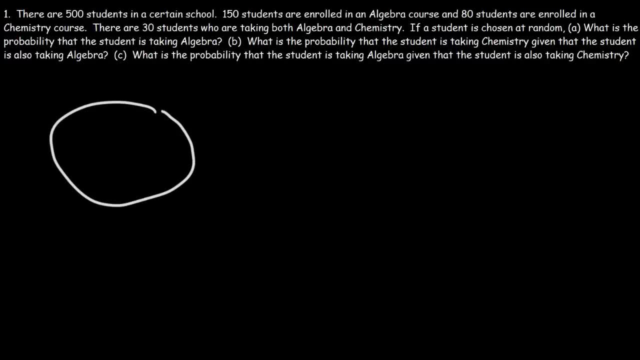 diagram. So we're going to draw two circles, with the circles intersecting each other. Let's put A for algebra and C for chemistry. So there's 150 students taking algebra and there's 80 students taking chemistry. There's 30 taking both. 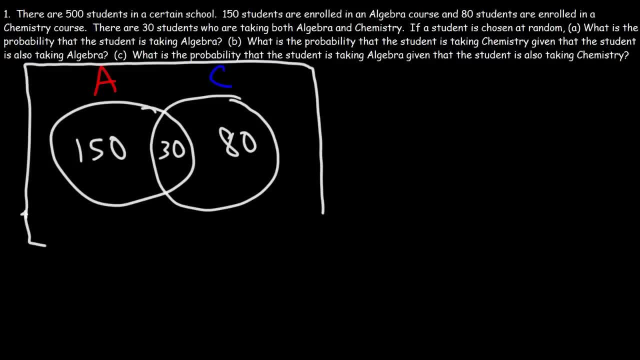 And in this school there's a total of 500 students. So what is the probability that the student is taking algebra? So there's 150 students taking algebra out of a total of 500 students. So this becomes 15 over 50.. 15 is 5 times 3.. 50 is. 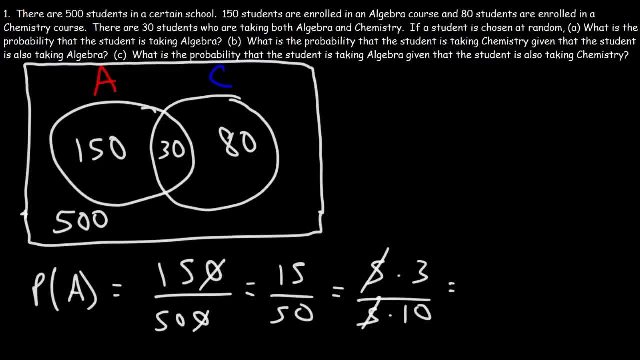 5 times 10.. And so the probability of selecting an algebra student is 3 over 10,, which is 0.3 or 30%. Now what about part B? What is the probability that the student is taking chemistry, given that the student is also taking algebra? 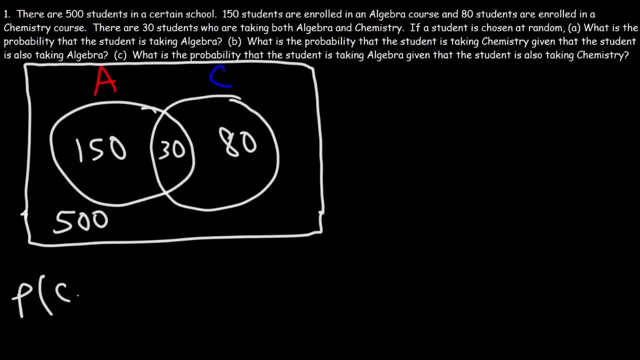 So this is a conditional. This is a conditional probability problem. So we're going to find the probability of getting C, given that the student is taking algebra or given A. So how much of C is in A? Think of it that way: We have 30 of C that is in A, So it's. 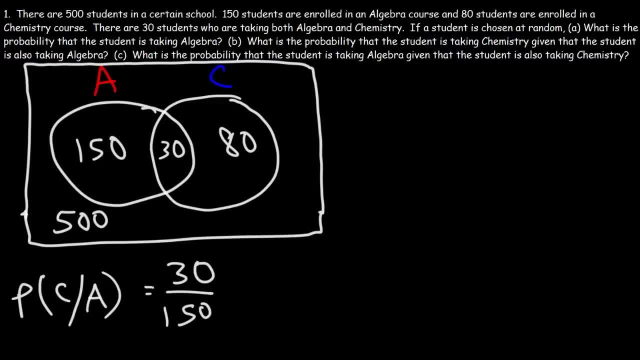 going to be 30 out of 150.. Now, for those of you who prefer to use the formula, you can use the formula. This is going to be the probability of getting C and A divided by the probability of getting A. So the probability of getting C and A, the probability that a student is taking algebra. 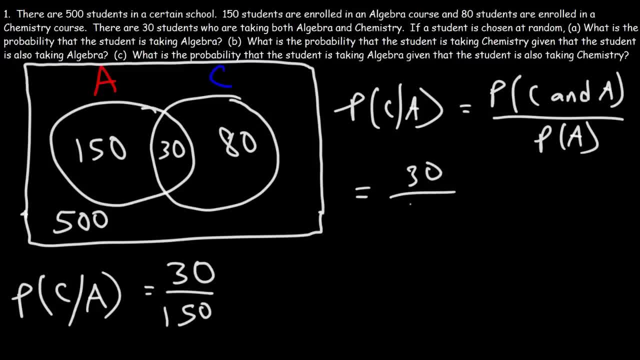 and chemistry is 30 out of a total of 500 students. The probability of a student taking algebra, that is, the probability of A, is 150 out of 500, which we calculated earlier, And so multiplying the top and the bottom by 500, you can see we're going to get the 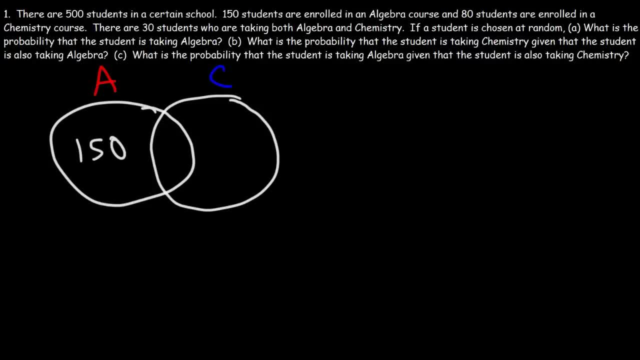 So there's 150 students taking algebra And there's 80 students taking chemistry, There's 30 taking both And in this school there's a total of 80 students taking chemistry Of 500 students. So what is the probability that the student is taking algebra? 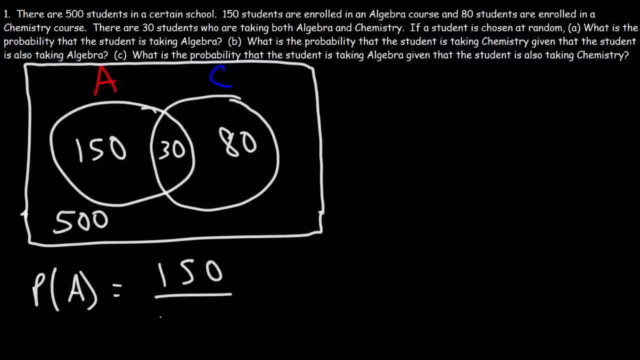 So there's 150 students taking algebra out of a total of 500 students. So this becomes 15 over 50.. 15 is 5 times 3,, 50 is 5 times 10.. And so the probability of selecting an algebra student is 5 times 10.. 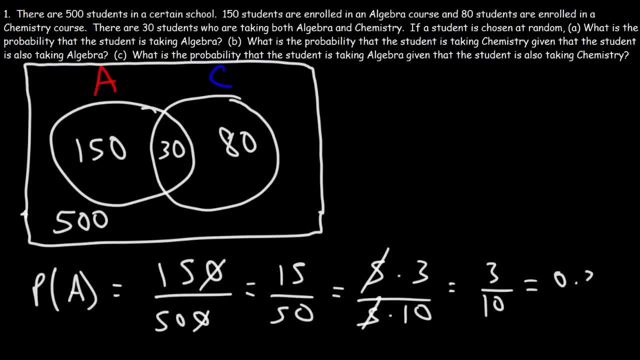 And so the probability of selecting an algebra student is 15 over 50.. a student is 3 over 10, which is 0.3 or 30%. Now what about part B? What is the probability that the student is taking chemistry, given that the student is? 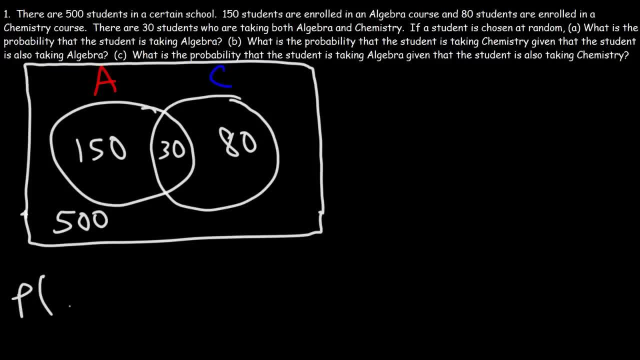 also taking algebra. So this is a conditional probability problem. So we're going to find the probability of getting C, given that the student is taking algebra or given A. So how much of C is in A? Think of it that way: We have 30 of C that is in A, so it's going to be 30 out of 150. 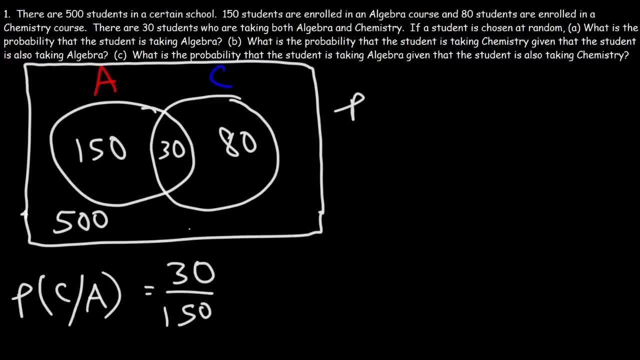 Now for those of you who prefer to use the formula, this is going to be The probability of getting C and A divided by the probability of getting A. So the probability of getting C and A, the probability that a student is taking algebra and chemistry- is 30 out of a total of 500 students. 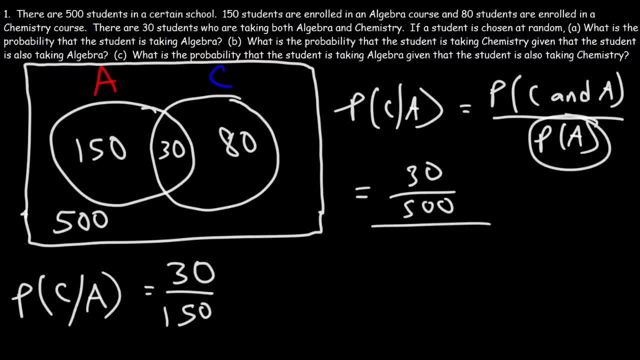 The probability of a student taking algebra, that is, the probability of A, is 150 out of 150 students, 150 out of 500, which we calculated earlier, And so multiplying the top and the bottom by 500, you can see we're going to get the. 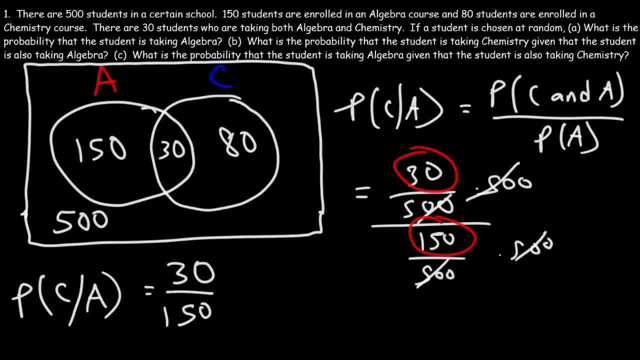 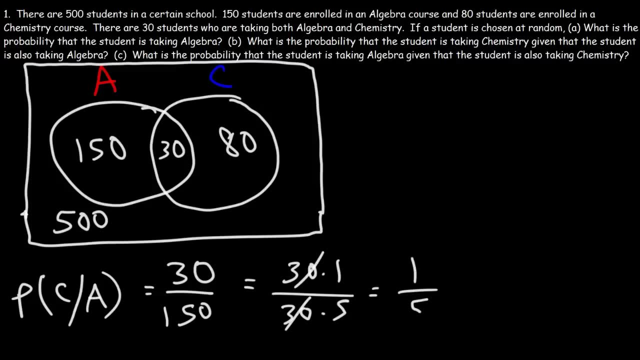 same answer: It's going to be 30 over 150.. So let's simplify: 30 over 150.. 30 is 30 times 1.. 150 is 30 times 5.. Okay, So the probability is going to be 1 over 5, which is 1 divided by 5 is 0.2.. 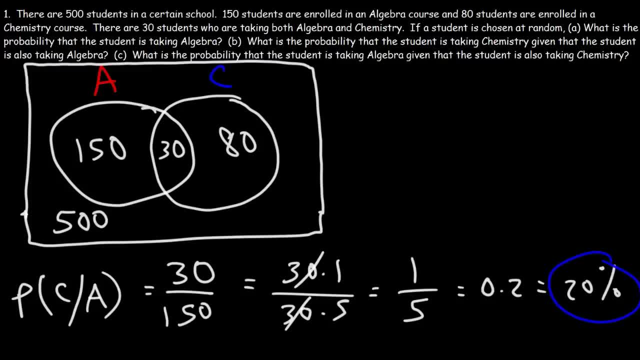 So there's a 20% chance of selecting a student who is taking chemistry, given that they're taking algebra. Now let's talk about what this means. Out of all of the 150 algebra students in this school, 20% of them is taking chemistry. 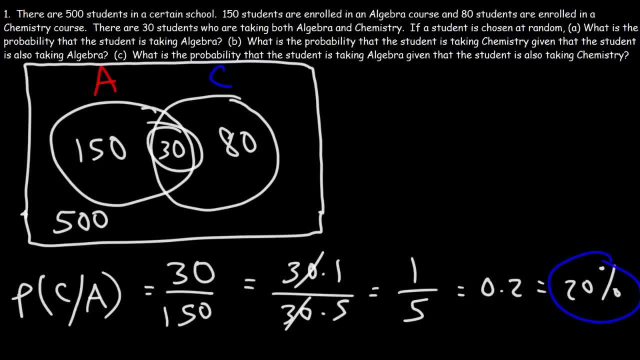 Right, 20% of 150 is 30.. Now let's move on to the last part of this problem, Part C. What is the probability that the student is taking algebra, given that the student is also taking chemistry? So, going back to part B, we said the probability of getting C, given A was 1 over 5.. 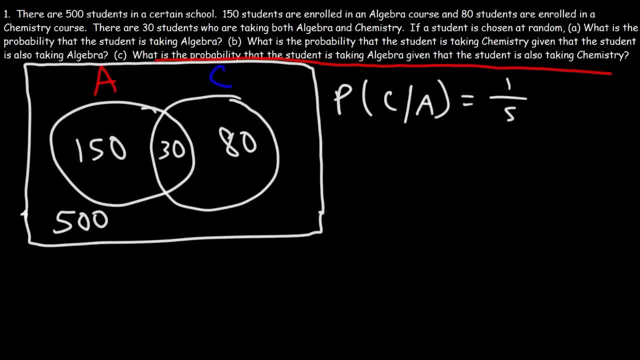 And part C was 1 over 5.. What's that? It's still 1 over 5.. It's still 1 over 5.. And we also said the probability of getting A equals 1 over 5.. Now, in this problem, we're looking for something different. 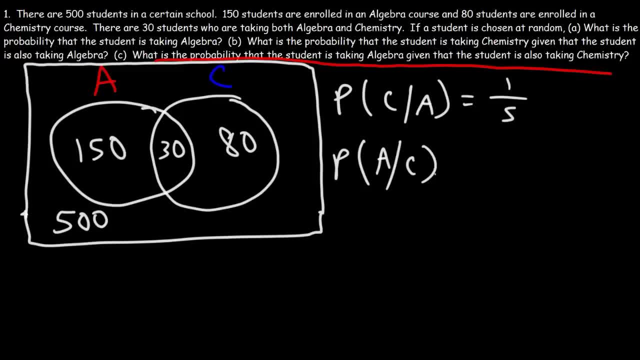 We're looking for the probability of A given C, and these are not the same. So what is the probability of selecting a student who has taken algebra, given that that student is taking chemistry as well? So how much of A is in C? 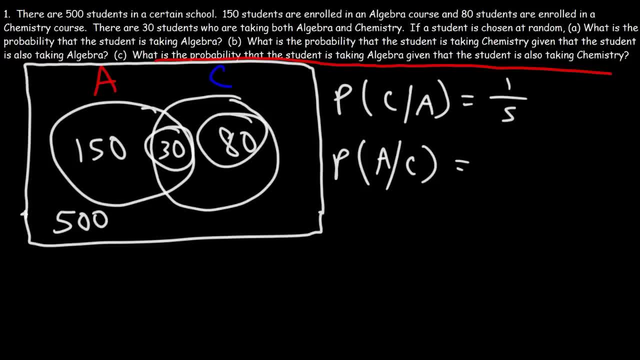 Notice that we have 30 of A, that is in basically 80 of C. So this is going to be 30 over 80, which we can reduce that to 3 over 8.. So out of the 80 students who are taking chemistry, 30 of them is taking algebra. 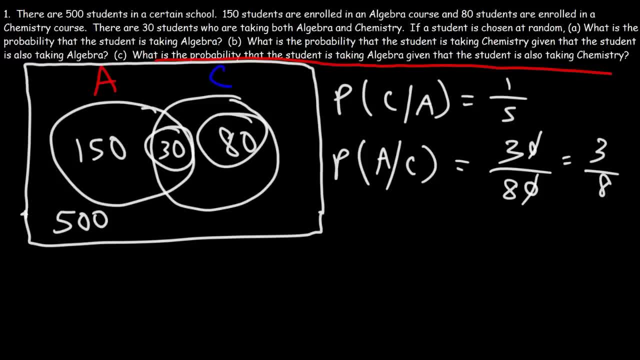 So the probability of selecting a student that is taking algebra, given that they're taking chemistry, is 3 out of 8.. And so that's a simple way in which you can do algebra Conditional probability calculations. Let's move on to the next question. 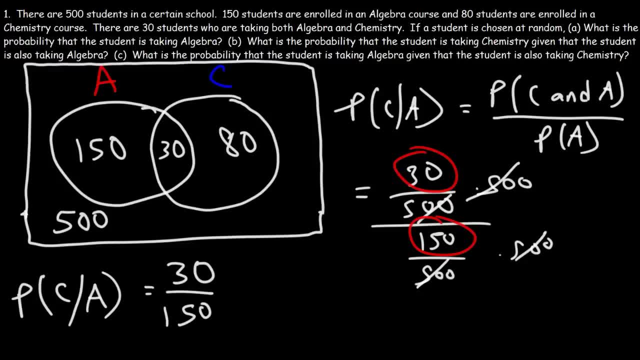 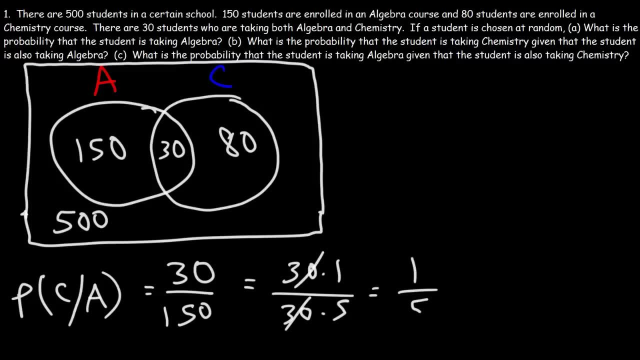 same answer: It's going to be 30 over 150.. So let's simplify: 30 over 150.. 30 is 30 times 1.. 150 is 30 times 5.. So the probability is going to be 1 over 5.. 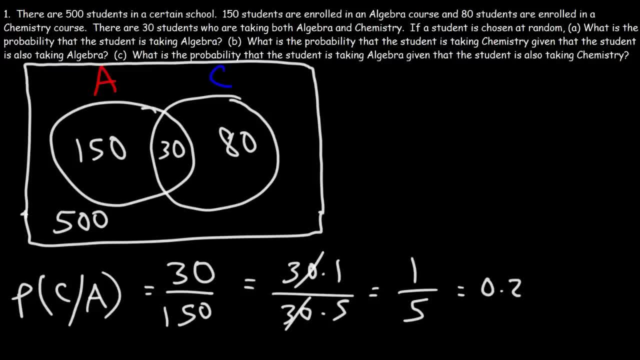 Which is 1 divided by 5, is 0.2.. So there's a 20% chance of selecting a student who is taking chemistry, given that they're taking algebra. Now let's talk about what this means. Out of all of the 150 algebra students in this school, 20% of them is taking chemistry. 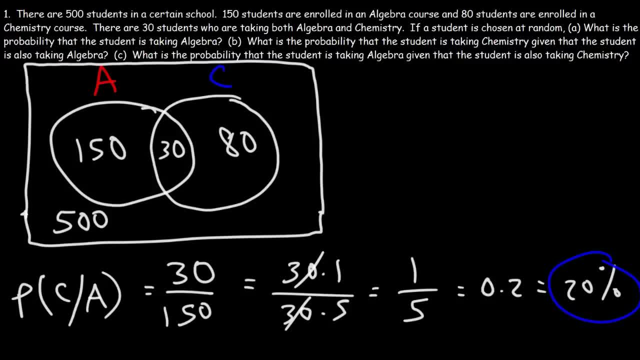 20% of 150 is 30.. Now let's move on to the last part of this problem, part C. What is the probability that the student is taking algebra, given that the student is also taking chemistry? So, going back to part B, we said the probability of getting C, given A was 1 over 5.. 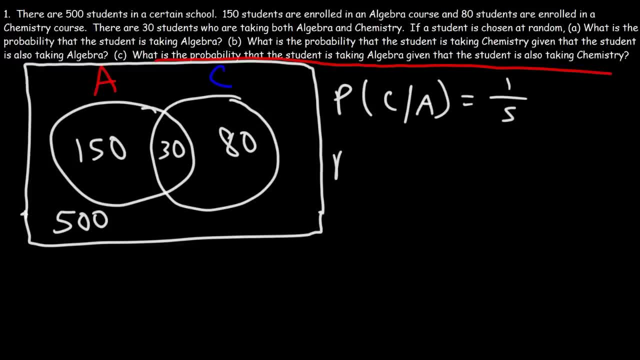 Now, in this problem, we're looking for something different. We're looking for the probability of A given C, And these are not the same. So what is the probability of selecting a student who is taking algebra, given that that student is taking chemistry as well? 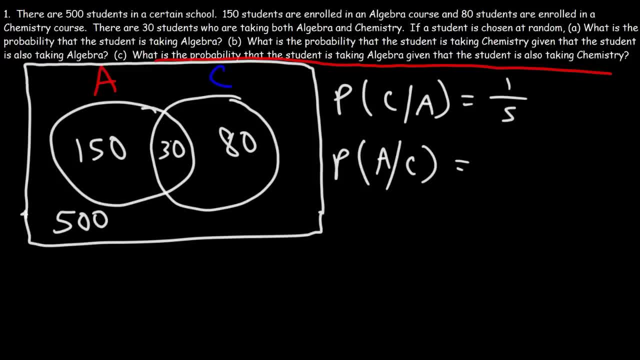 So how much of A is in C? Notice that we have 30 of A, that is in basically 80 of C. So this is going to be 30 over 80, which we can reduce that to 3 over 8.. So out of the 80 students who are taking chemistry, 30 of them is taking algebra. 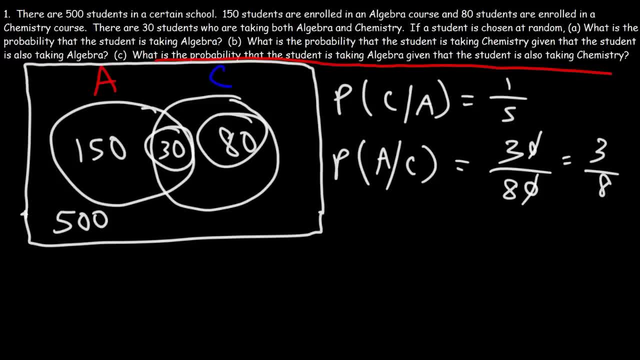 So the probability of selecting a student that is taking algebra- given that they're taking chemistry- is 3 out of 8.. And so that's a simple way in which you can do conditional probability calculations. Let's move on to the next question. 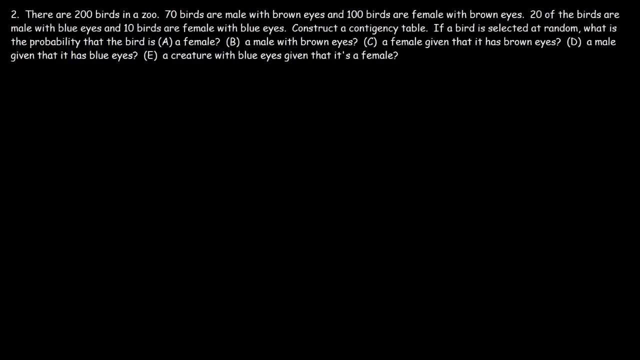 There are 200 birds in a zoo. Seventy birds are male with brown eyes and 100 birds are female with brown eyes. Twenty of the birds are male with blue eyes and 10 birds are female with blue eyes. Construct a contingency table. 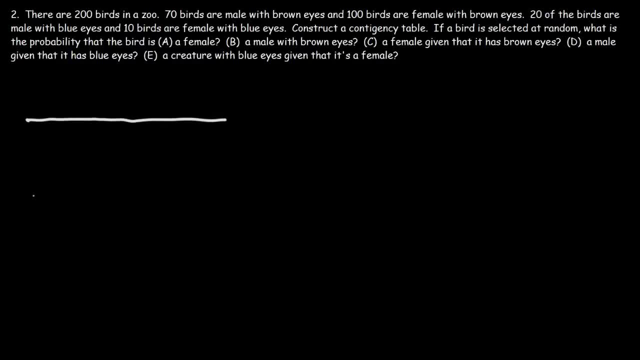 So let's begin by doing that first. So on the left we're going to have the gender, So it's either male or female, And at the top we're going to put the color of the eyes: either blue eyes or brown eyes. 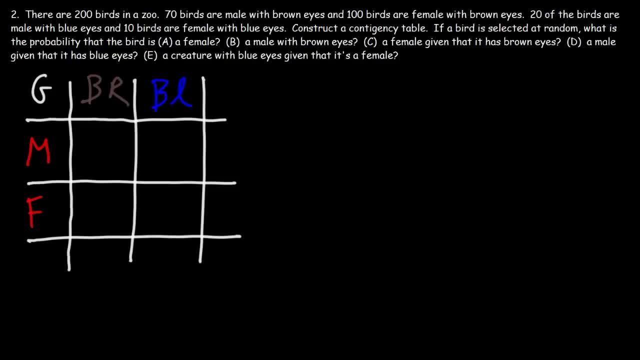 Let me pick a different color for this, And at the sides we're going to put the totals. So 70 birds are male with brown eyes, So let's put a 70 here. A hundred birds are female with brown eyes. Twenty birds are male with blue eyes. 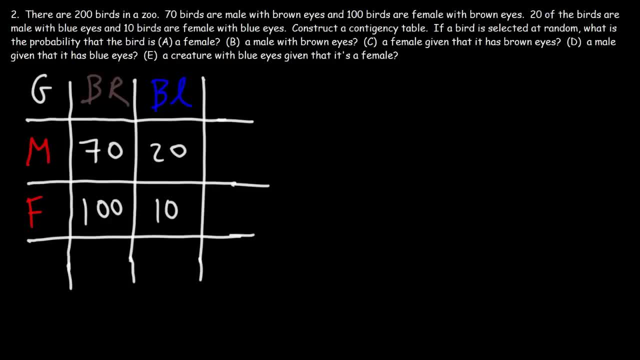 Ten birds are female with blue eyes. So we're going to put the totals And at the sides, we're going to put the totals. So what's the total number of males? Seventy plus 20 is 90. Now the total number of female birds is going to be 100 plus 10, which is 110.. 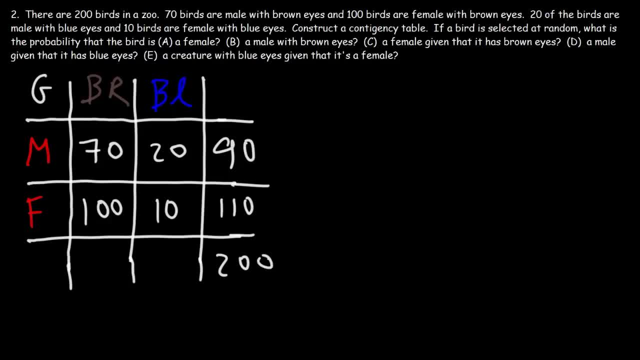 So adding these two will give us a total of 200 birds in this zoo. Now let's add these numbers, So the total number of birds with brown eyes is 170.. The total number of birds with blue eyes is going to be 30.. 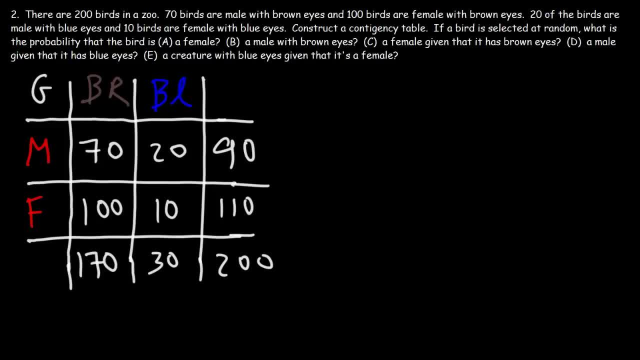 And we can see that 170 plus 30 is 200.. So now that we've filled out the contingency table, let's answer some questions. If a bird is selected at random, what is the probability that the bird is a female? So let's start with that. 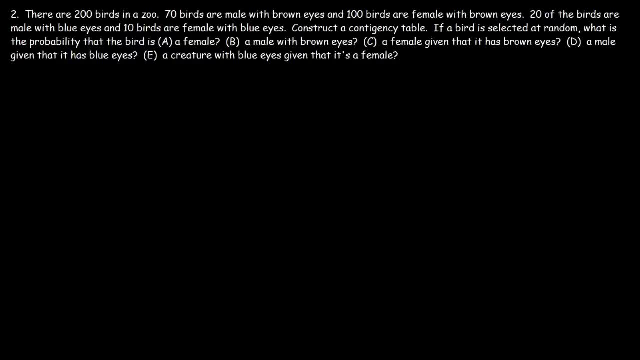 There are 200 birds in a zoo. 70 birds are male with brown eyes and 100 birds are female with brown eyes. 20 of the birds are male with blue eyes and 10 birds are female with blue eyes. Construct a contingency table. 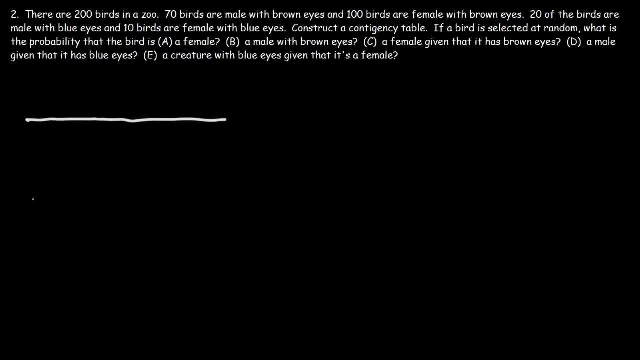 So let's begin by doing that. So we're going to start by doing that first. So on the left we're going to have the gender, So it's either male or female, And at the top we're going to put the color of the eyes. 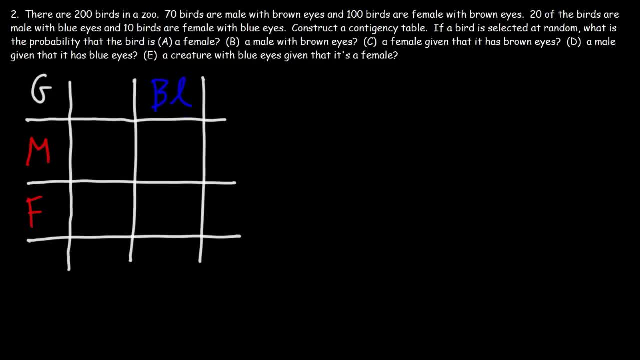 Either blue eyes or blue eyes, Blue eyes or brown eyes. Let me pick a different color for this, And at the sides we're going to put the totals. So 70 birds are male with brown eyes, So let's put a 70 here. 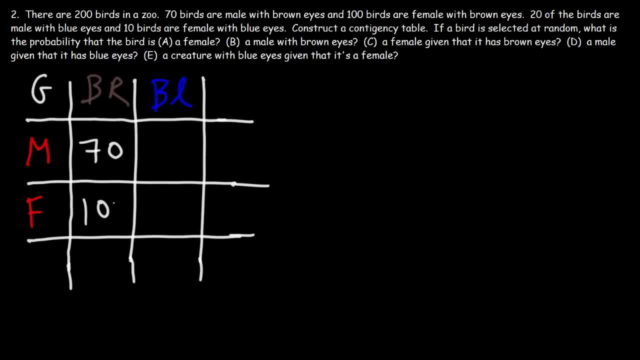 100 birds are female with brown eyes. 20 birds are male with blue eyes, 10 birds are female with blue eyes. So what's the total number of males? 70 plus 20 is 90.. Now the total number of female birds is going to be 100 plus 10, which is 110. 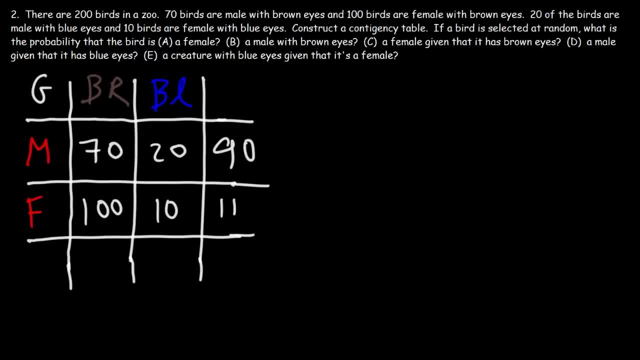 So adding these two will give us a total of 200 birds in this zoo. Now let's add these numbers, So the total number of birds with brown eyes is 3,000.. So 30 are female And 10 are male. 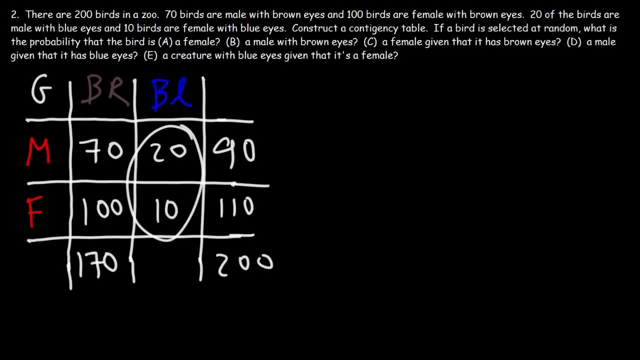 is 170.. The total number of birds with blue eyes is going to be 30. We can see that 170 plus 30 is 200.. So now that we filled out the contingency table, let's answer some questions. If a bird is selected at random, what is the? 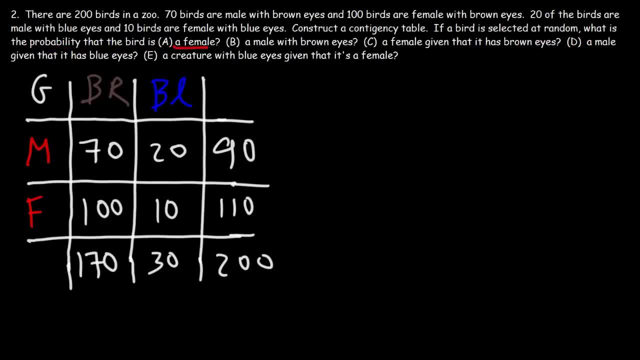 probability that the bird is a female, So let's start with that. So what's the probability of getting an F? So there's 110 birds that are female out of a total of 200 birds in the zoo, So the probability is going to be 110 over 200.. 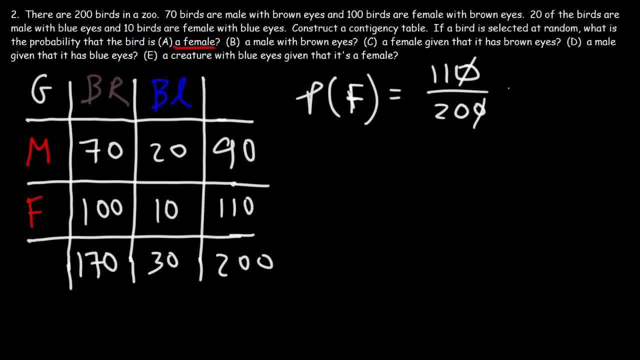 If we divide both numbers by 10, by getting rid of a zero, the probability is 11 over 20, which is 0.55, or A 55% chance of selecting a female bird. Now what about selecting a bird that is a male with brown eyes? 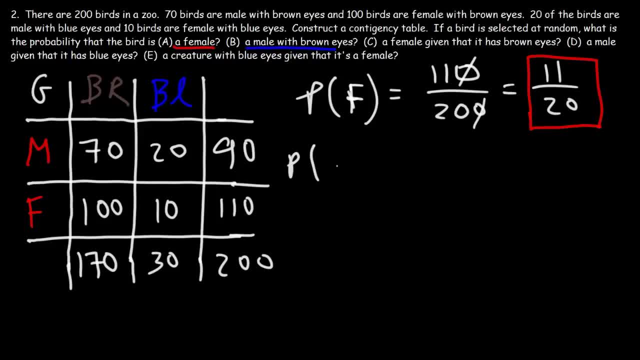 So this is not a conditional probability question. We're looking for a bird with two characteristics: It has to be a male and it has to have brown eyes. So there's 70 birds that are both male and with brown eyes Out of a total of 200 birds. 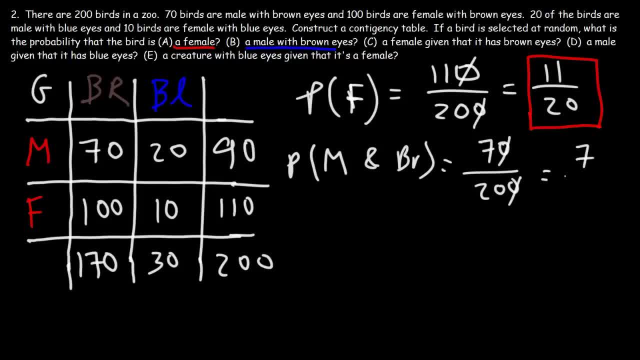 So the probability is going to be 7 out of 20, which is 0.35, which corresponds to a 35% chance of selecting such a bird. Now let's move on to part C. So what is the probability that the bird is a female, given that it has brown eyes? 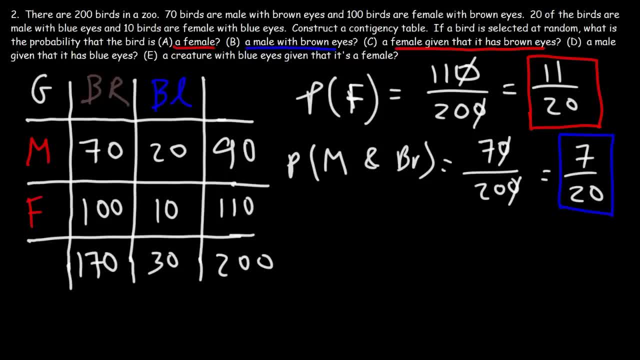 So now we're dealing with a conditional probability question. So what is the probability that we're going to get F given B R? So, to do it the easy way, think about this question: How much of F is in B R? So, out of all the birds with brown eyes, how much is female? 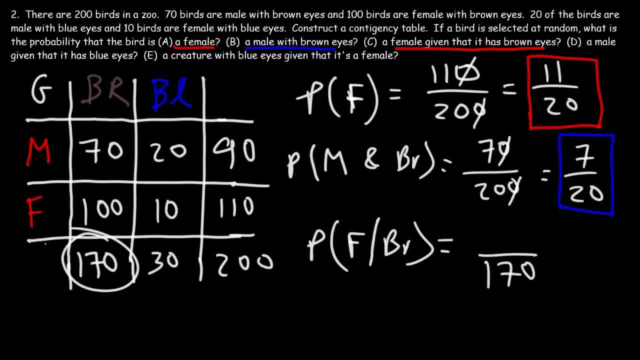 So there's 170 birds with brown eyes. A hundred of those birds are female, So it's going to be 100 out of 170, which reduces to 10 over 17.. Now if we divide 10 by 17,, 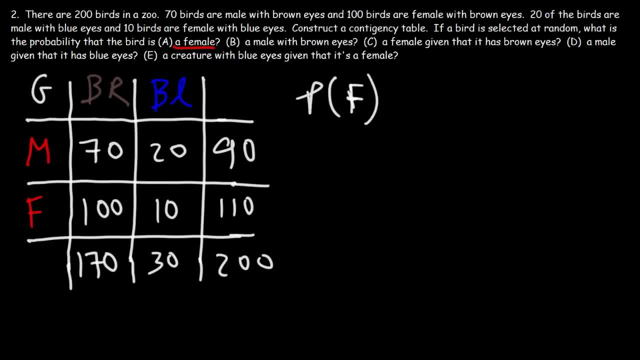 So what's the probability of getting F? Okay, Okay, Okay. So you have 110 birds that are female out of a total of 200 birds in the zoo, So the probability is going to be 110 over 200.. If we divide both numbers by 10, by getting rid of a zero, the probability is 11 over. 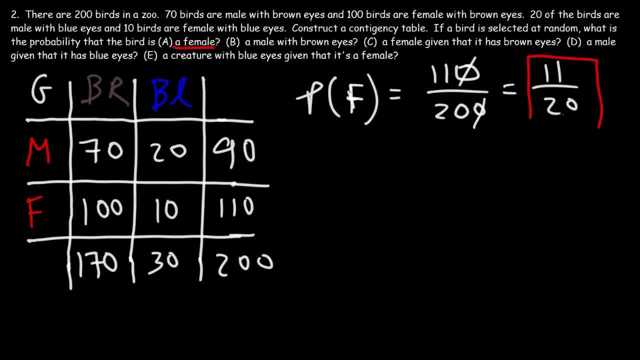 20,, which is 0.55, or a 55% chance of selecting a female bird. Now, what about selection? Now, what about selecting a bird that is a male with brown eyes? So this is not a conditional probability question. 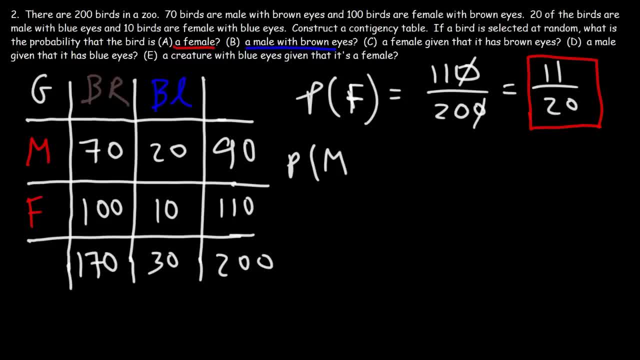 We're looking for a bird with two characteristics: It has to be a male and it has to have brown eyes. So there's 70 birds that are both male and with brown eyes out of a total of 200 birds. So the probability is going to be 7 out of 20, which is 0.35,. 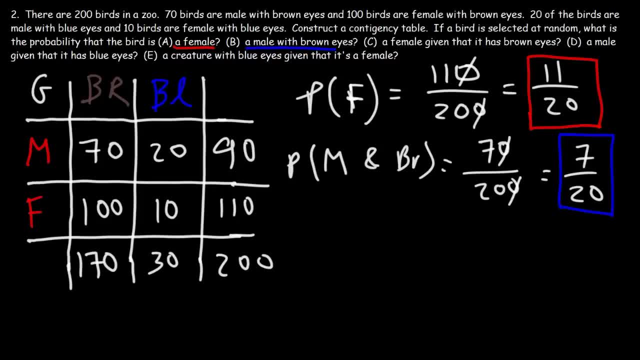 which corresponds to a 35% chance of selecting such a bird. Now let's move on to part C. So what is the probability that the bird is a female, given that it has brown eyes? So now we're dealing with a conditional probability question. 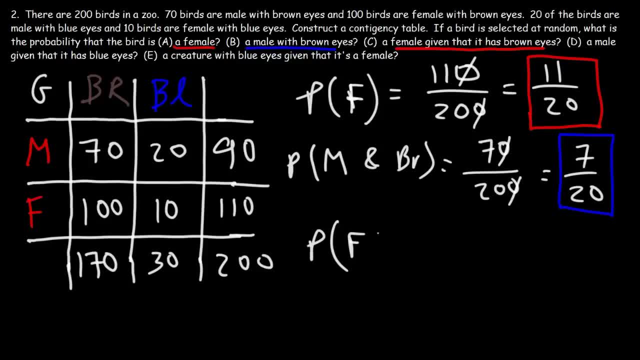 So what is the probability that the bird is a female, given that it has brown eyes? We're going to get F given BR. So, to do it the easy way, think about this question: How much of F is in BR? So, out of all the birds with brown eyes, how much is female? 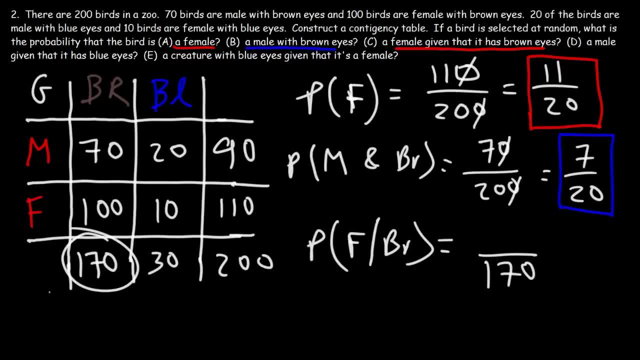 So there's 170 birds with brown eyes. A hundred of those birds are female, So it's going to be 100 out of 170.. Which reduces to 10 over 17.. Now if we divide 10 by 17,, that's going to be 0.588.. 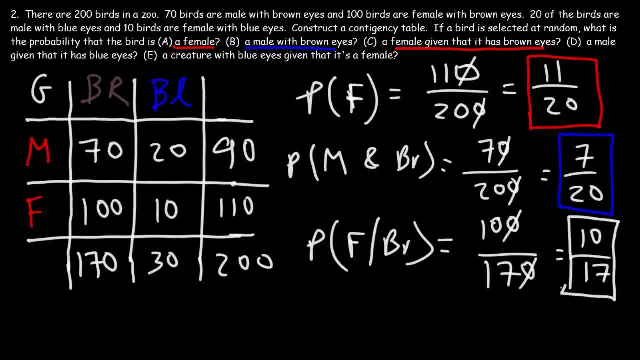 So let's talk about what this means. That means there's a 58.8% chance of selecting a bird that is a female, given that the bird has brown eyes. So, out of all of that, there's a 58.8% chance of selecting a bird that is a female, given that the bird has brown eyes. 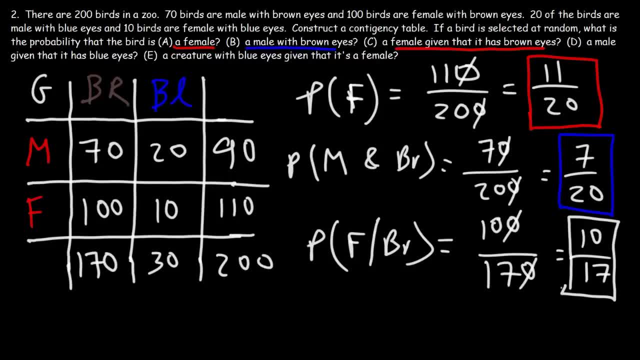 that's going to be 0.588.. So let's talk about what this means. That means there's a 58.8% chance of selecting a bird that is a female, given that the bird has brown eyes. So, out of all of the 170 birds with brown eyes, 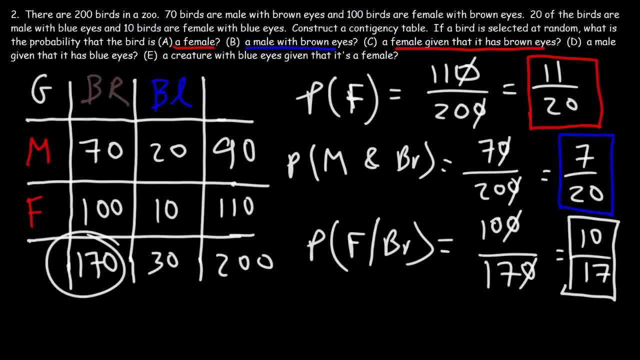 58.8% of those birds are female, So that's what that means. Now let's move on to part D. What is the probability that the bird is a male, given that it has blue eyes? So what's the probability of M, given B, L? 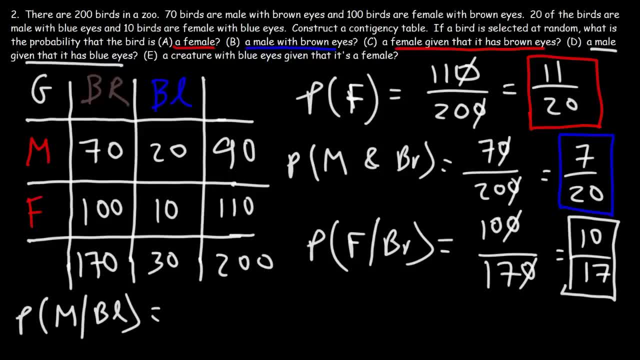 So how much of M is in B L? There's 20 of M and 30 of B L, So there's a total of 30 birds with blue eyes, 20 of which are male. So the probability of selecting a male bird, given that it has blue eyes, is 2 over 3.. 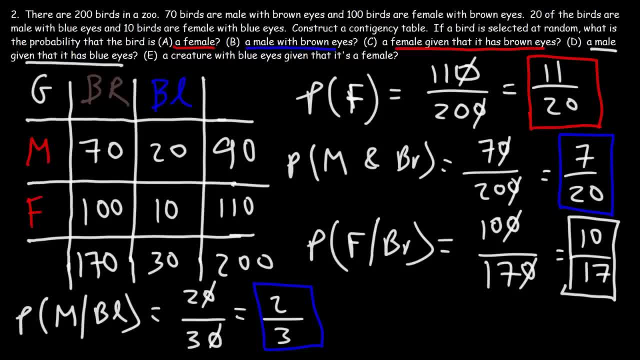 So, as you can see, it's really not that difficult when calculating conditional probability if you understand the principles behind it. Now, before we answer the last question, I just want to clear away a few things, because this page is getting crowded now. 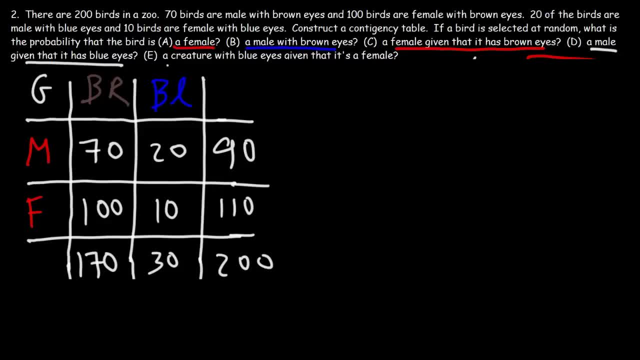 So the last part. What is the probability that the bird is a creature with blue eyes, given that it's a female? So what's the probability of B L given F? So how much of B L is in F? So there is 110 female birds, 10 of which contain blue eyes. 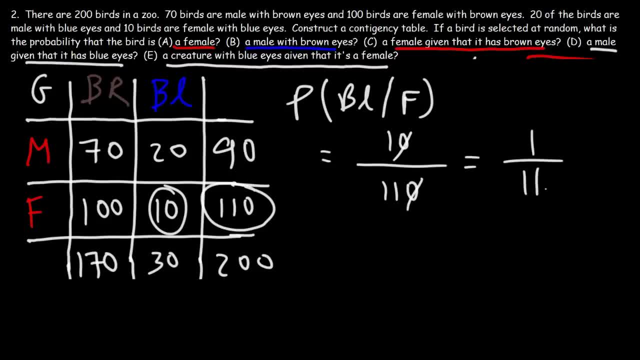 So the probability is going to be 1 over 11.. There's, out of all the 110 female birds, 10 of those have blue eyes, And so this is it. That's. all you got to do is 10 over 1, 10, which reduces to 1 over 11.. 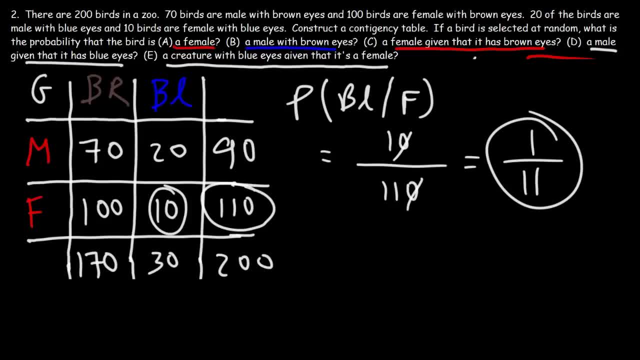 And let's turn that into a decimal value, So that's approximately 0.091,. if you round it, So there's a 9.1% chance of selecting a bird with blue eyes, given that it's a female. 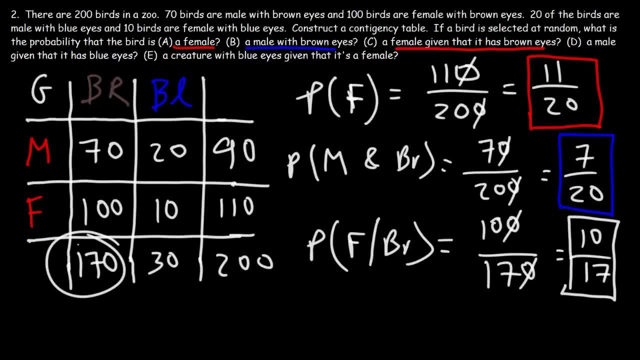 So, out of all of the 170 birds with brown eyes, 58.8% of those birds are female. So that's what that means. Now let's move on to part D. What is the probability that the bird is a male? 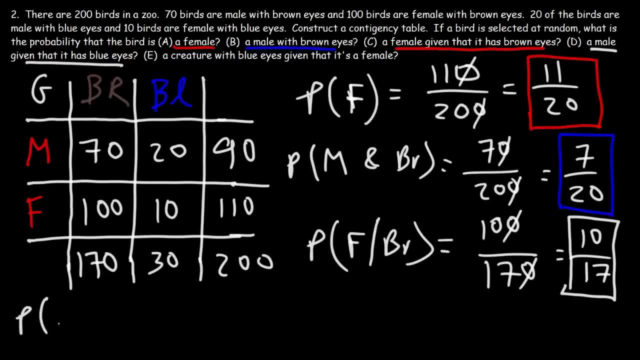 given that it has blue eyes. So what's the probability of M given BL? So how much of M is in BL? There's 20 of M And 30 of BL, So there's a total of 30 birds with blue eyes. 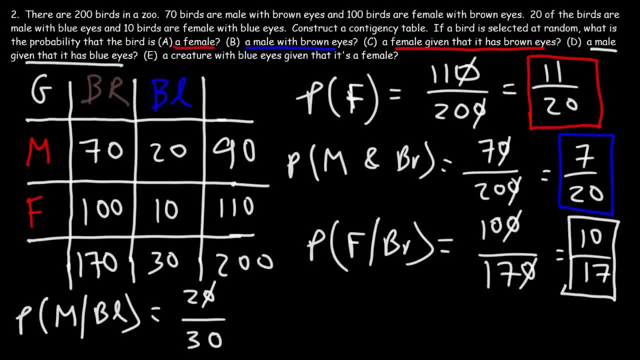 20 of which are male. So the probability of selecting a male bird, given that it has blue eyes, is 2 over 3.. So, as you can see, it's really not that difficult when calculating conditional probability, if you understand the principles behind it. 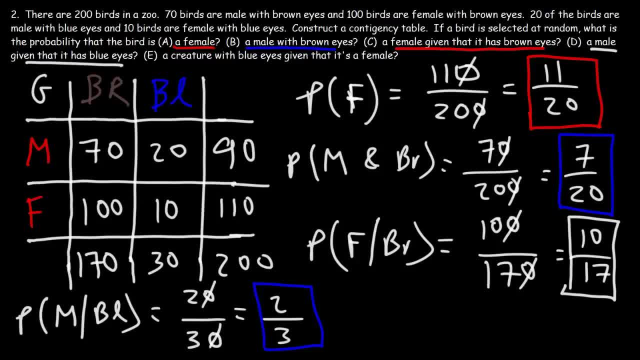 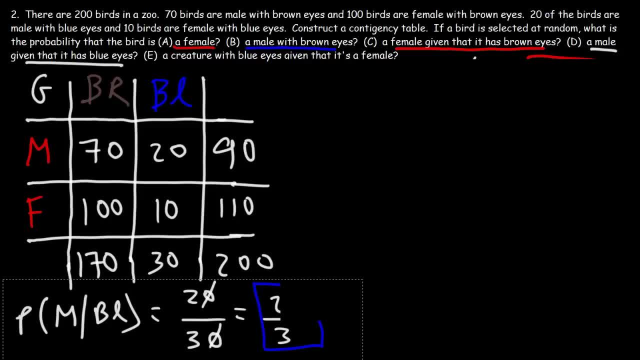 Dr David Judy. Now, before we answer the last question, I just want to clear away a few things, Because this page is getting crowded. now The last part: What are the probability that the bird is a creature with blue eyes, given that it's a female? 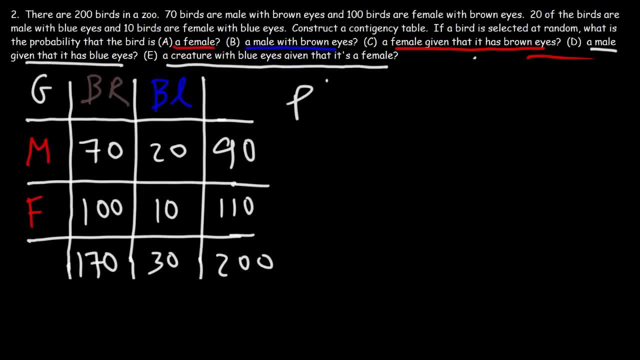 So what's the probability of BL given F? So how much of BL given f is 30%, so 30.3% G- This is the answer to turn again- is in F. So there is 110 female birds, 10 of which contain blue eyes. So the probability. 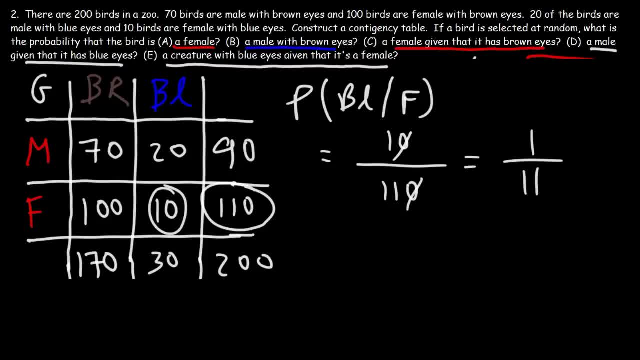 is going to be 1 over 11.. There's, out of all the 110 female birds, 10 of those have blue eyes, And so this is it. That's. all you got to do is 10 over 1, 10, which reduces to 1. 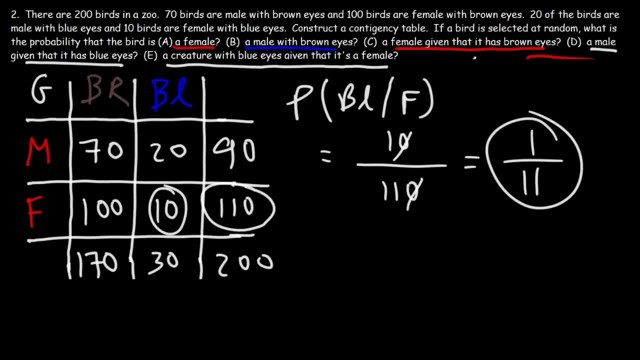 over 11.. And let's turn that into a decimal value, So that's approximately 0.091 if you round it. So there's a 9.1% chance of selecting a bird with blue eyes, given that it's a female.